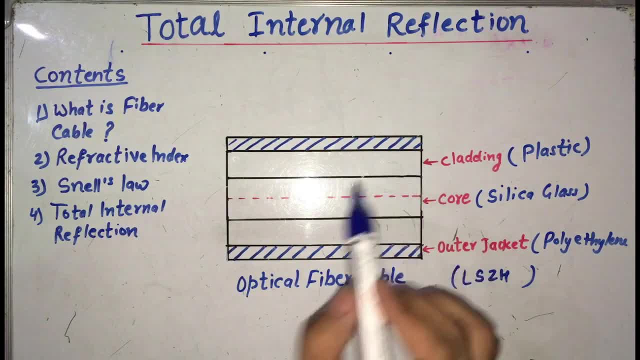 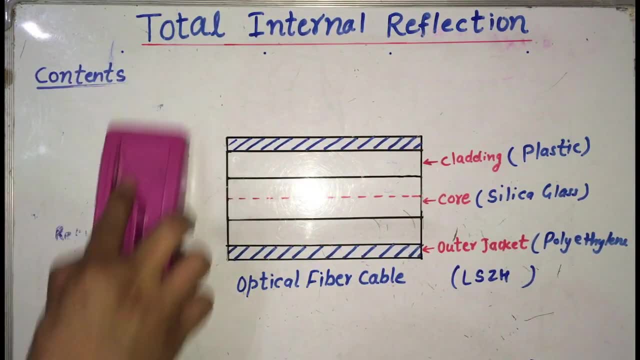 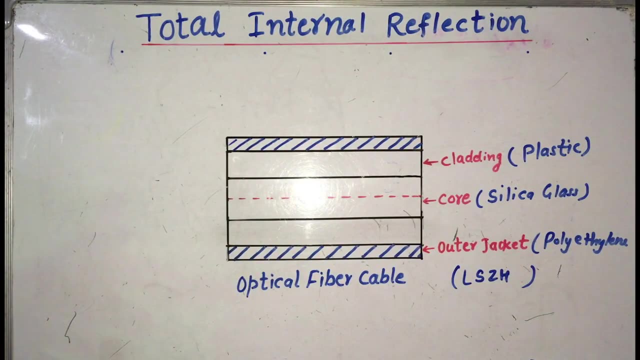 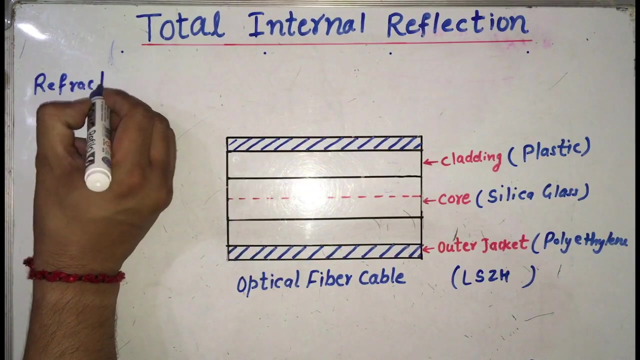 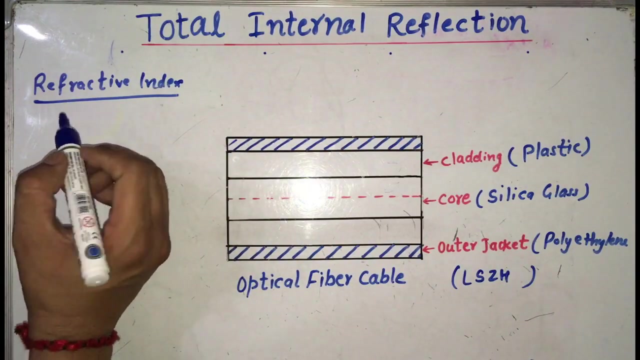 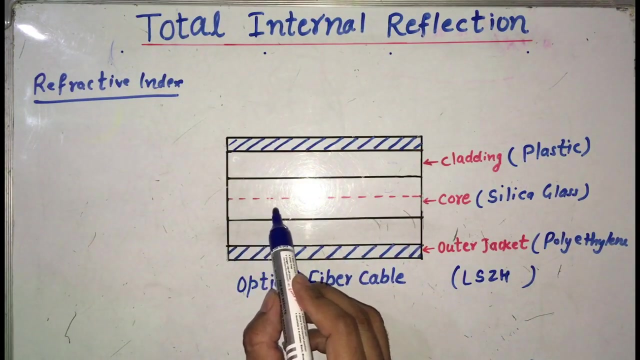 than core. So let us understand what is this refractive index? Now, refractive index, Okay, Refractive index of any material is a dimensionless number. It tells us about that: how fast light will travel through a material in respect to the? 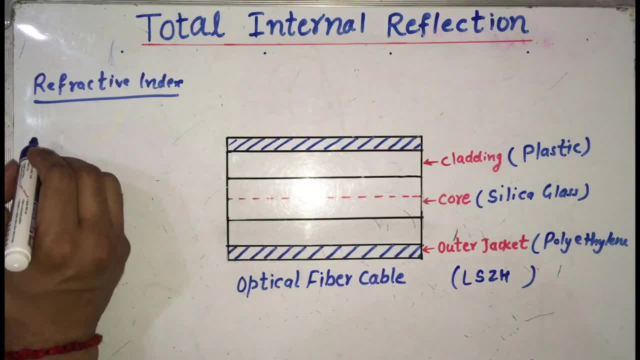 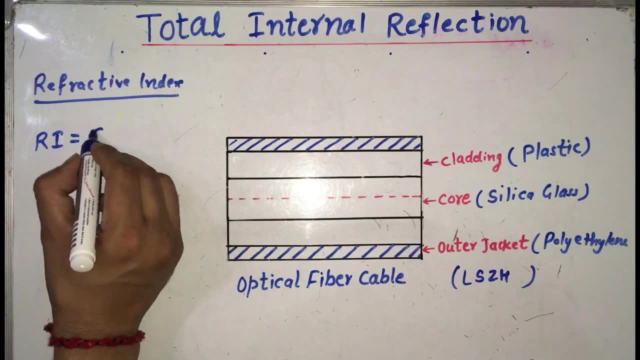 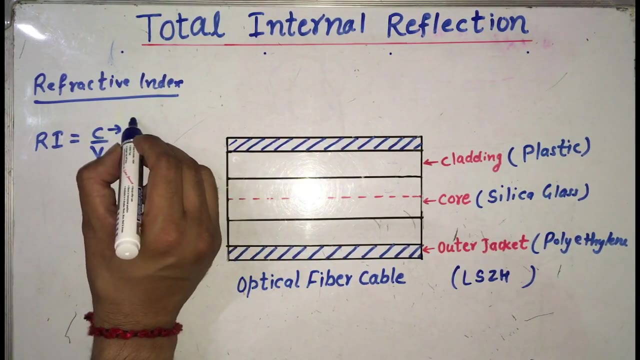 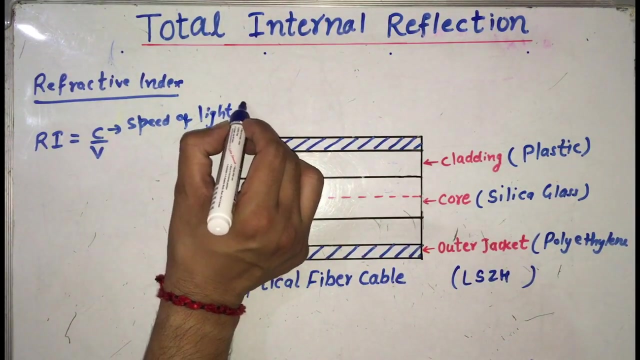 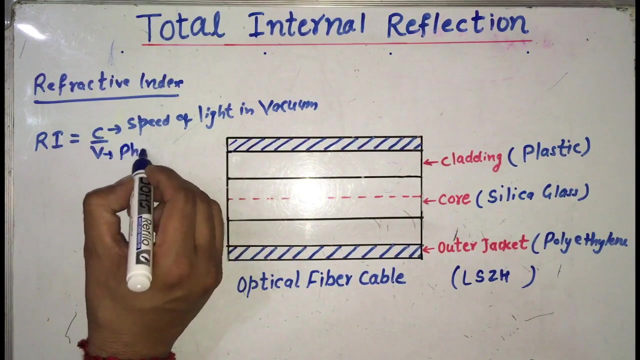 speed of light in vacuum. So we can calculate refractive index- let us say it is Ri refractive index- on any material by using this. This formula, Ri is equal to C upon V, where this C is speed of light in vacuum And V is the phase velocity of light in medium. 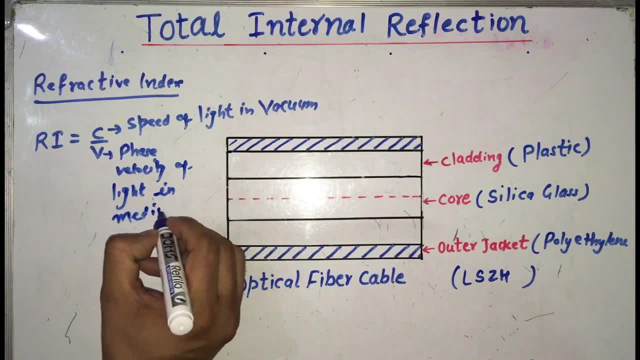 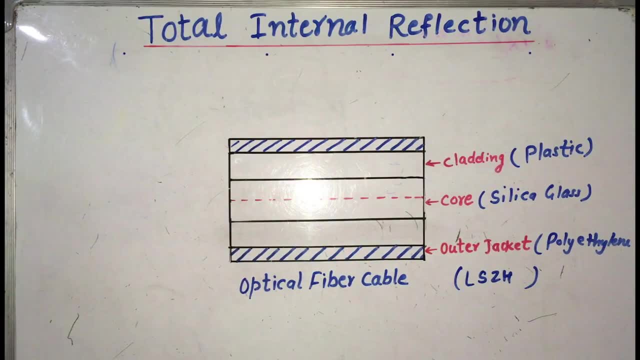 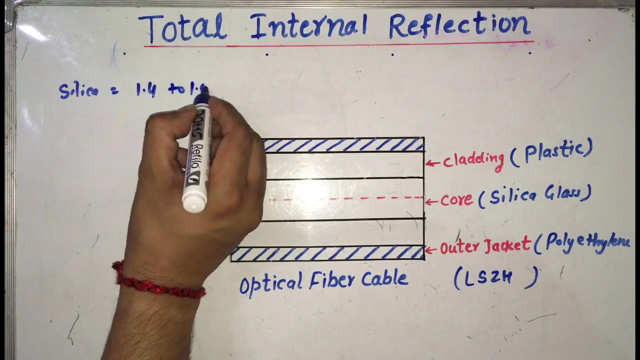 Okay, Okay, Okay, Okay, Okay, Okay. So this is called the refractive index of a material. So, for example, refractive index of silica is between 1.4 to 1.55.. So we can find out the speed of light in silica glass like this refractive index. 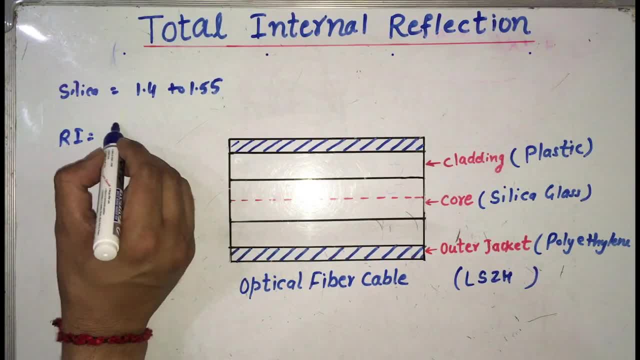 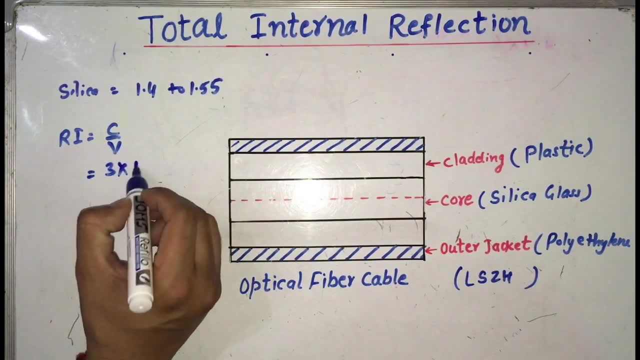 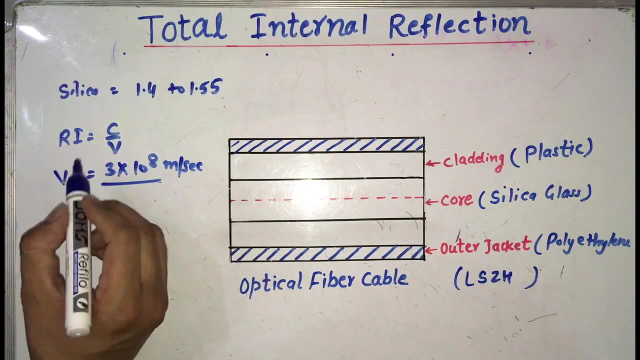 Okay, uh, refractive index was equal to c upon v. so we know that speed of light in vacuum is 3 into 10, raised to power, 8 meter per second, and divide by refractive index. refractive index lies between 1.4 to 1.55, for example, we can take a value 1.5. so phase velocity of 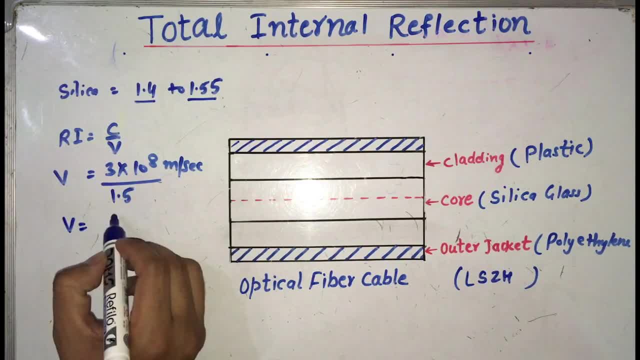 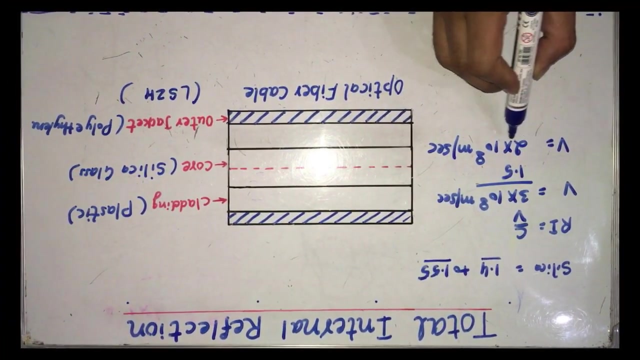 light in silica will be equal to 2 into 10, raised to power, 8 meters per second. so this is how we can find out the velocity of light in any of the material. so value of v indicates that light will travel with the speed of 2 into 10, raised to power, 8 meter per second in silica glass. 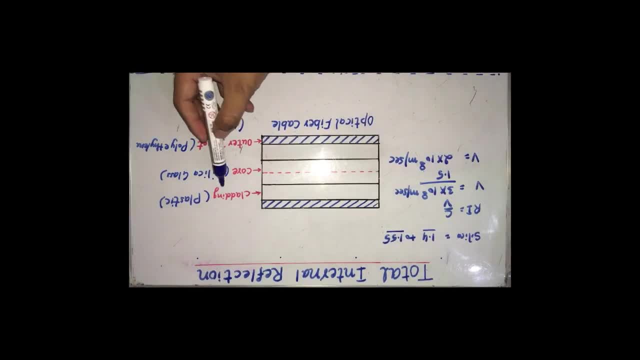 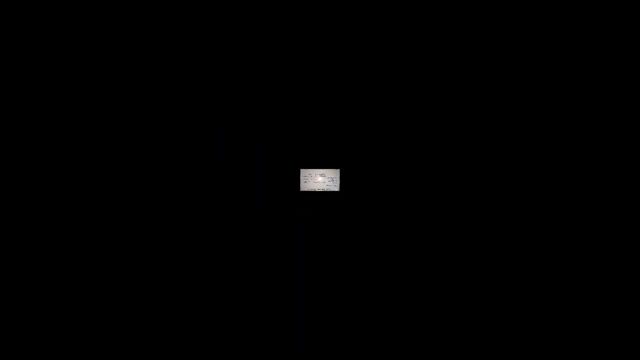 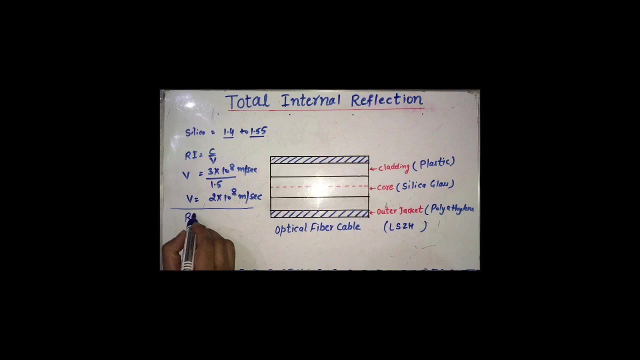 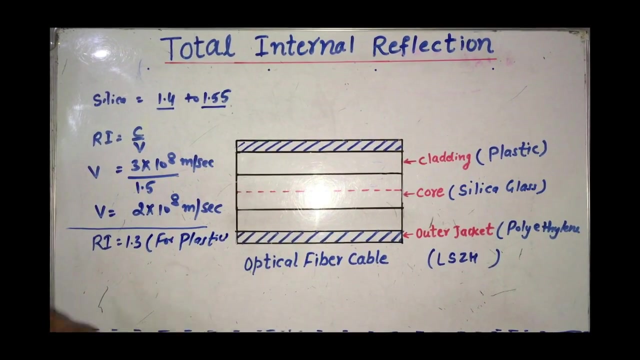 so Let us compare this with the speed of light in cladding. Now we know that cladding is made up of plastic material and refractive index for plastic is, for example, is 1.3 for plastic Now. so refractive index is equal to C upon V. 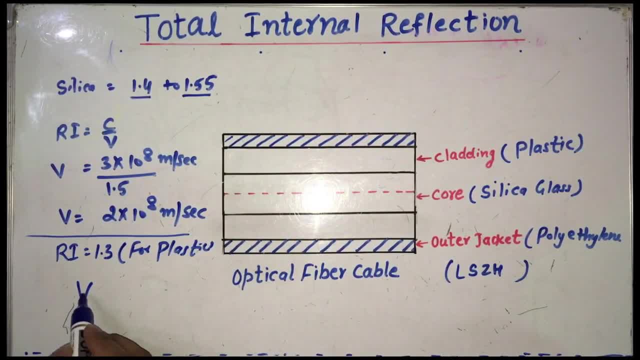 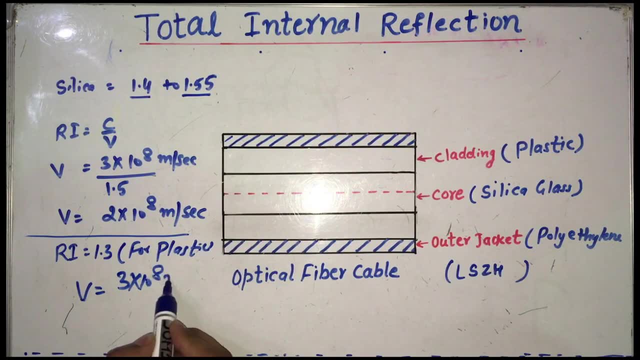 So from here, velocity of light phase velocity of light in plastic will be equal to 3 into 10, raised to power, 8 meter per second, divided by this 1.3.. So it will be something about 2.3 into 10, raised to power, 8 meter per second. 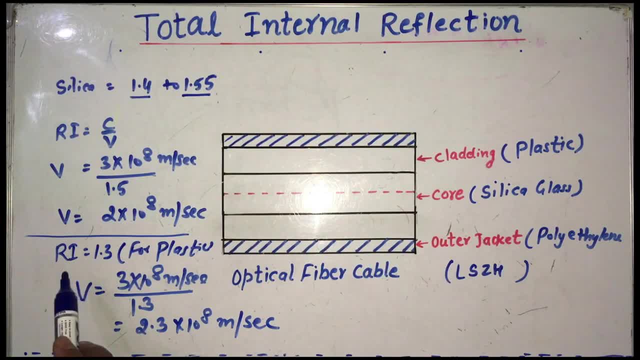 I hope now you can understand the effect of refractive index of a material On the speed of light into that material, Like we can say that in silica phase velocity of light will be 2 into 10, raised to power, 8 meter per second. 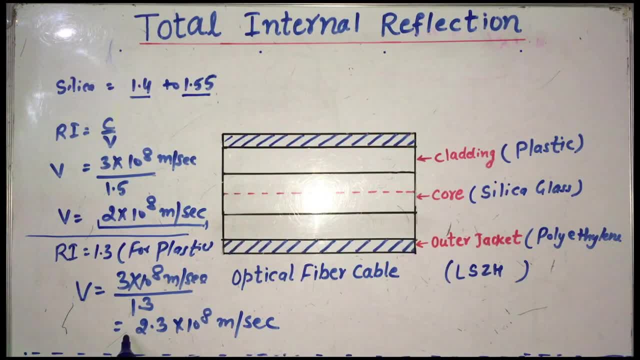 While it will be in plastic, which is a cladding material, it will be 2.3 into 10, raised to power, 8 meter per second. In both the cases, the speed of light will be slower than the speed of light in vacuum. 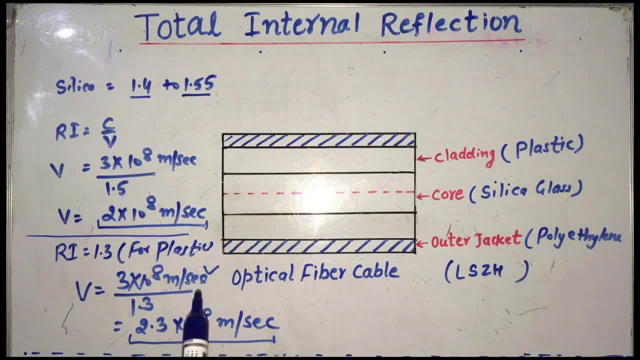 Now, this concept tells us about how fast light will travel from one medium to the other medium, So like if light falls upon this optical fiber cable, And this is the boundary where, on the inner side of it, silica glass is there. 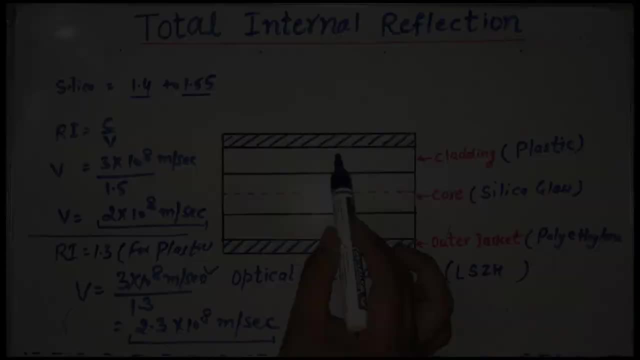 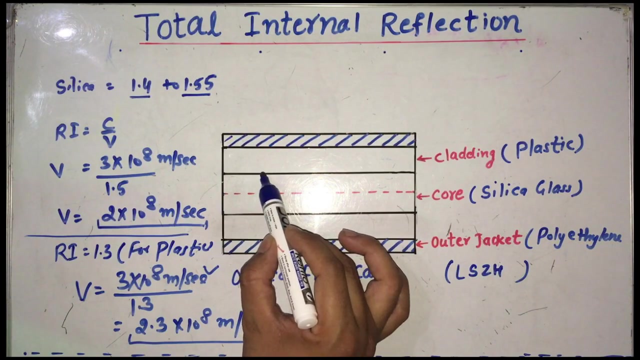 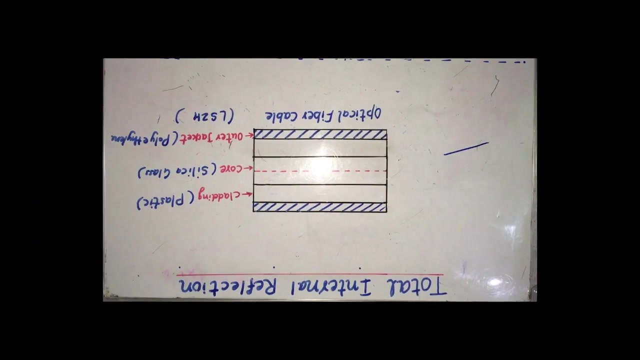 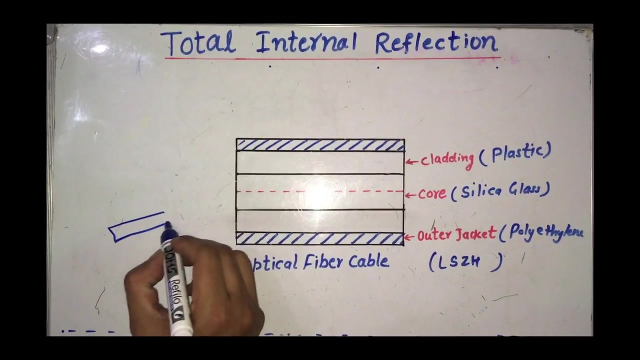 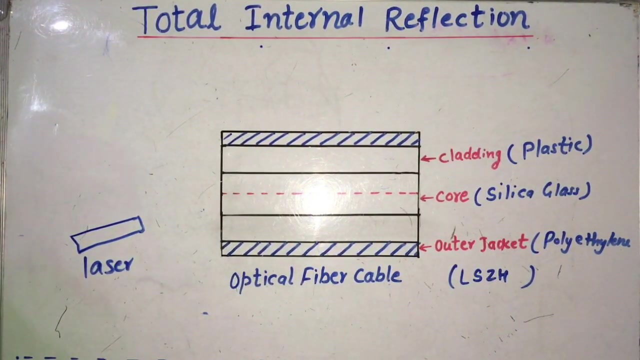 And in this layer, the material of this layer is plastic. So when light will fall upon this material and will try to cross this boundary, then speed of light will change. Now let us understand how total internal reflection works. Let us have a light source like this one- this is a laser, and a ray of light from this laser falls on the surface of this optical fiber cable. 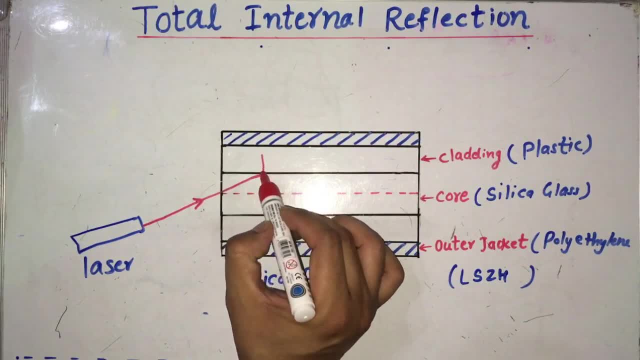 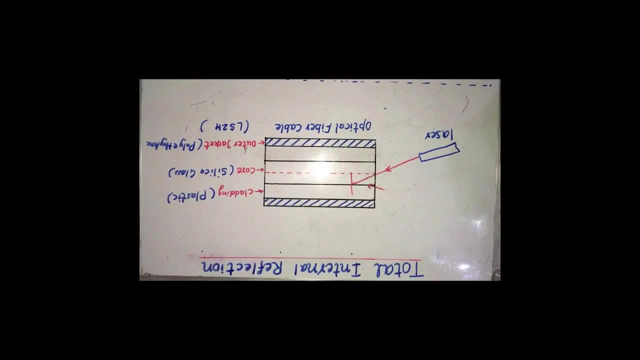 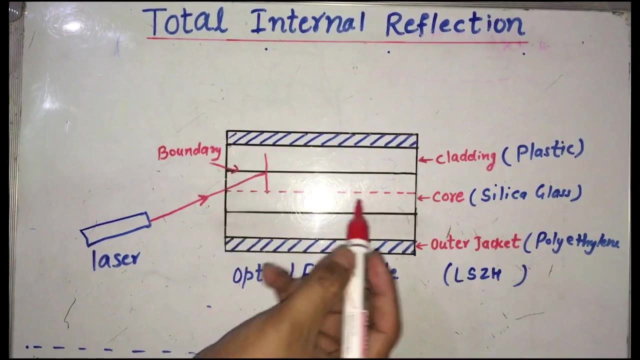 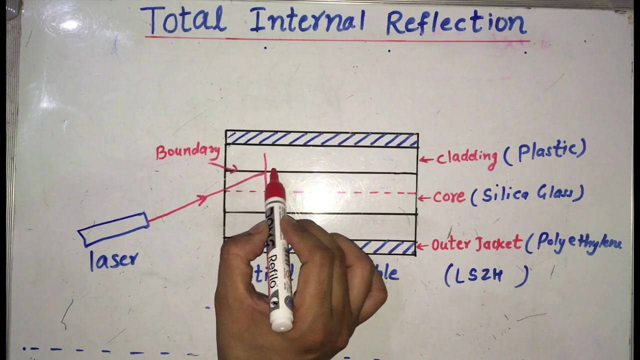 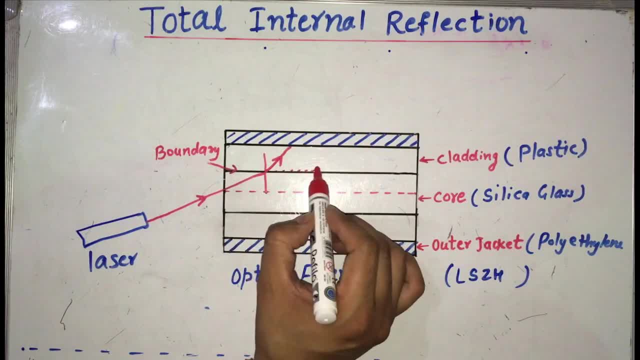 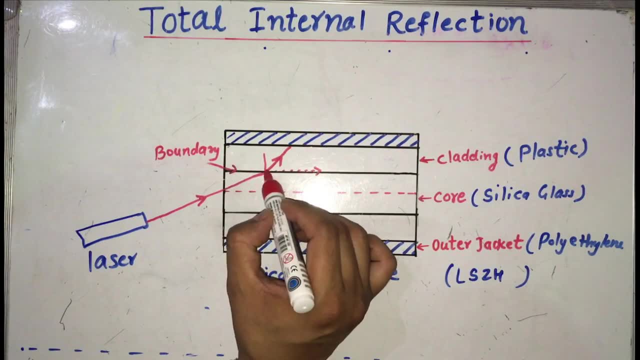 So when it strikes to the boundary of optical fiber cable, then there are three possibilities. So when it strikes to the boundary of optical fiber cable, then there are three possibilities parallel to the core cladding boundary. and third possibility is this ray of light will reflect back. 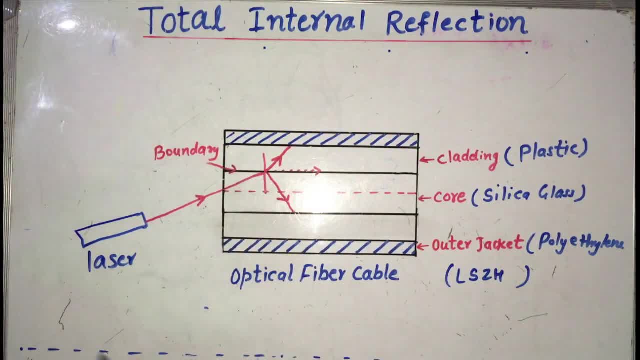 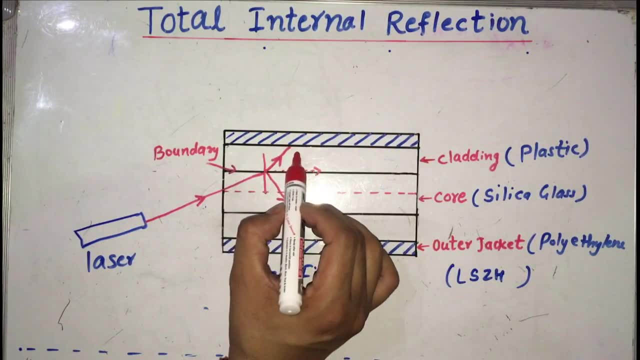 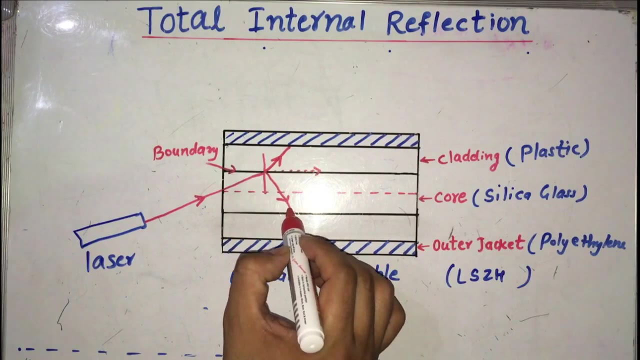 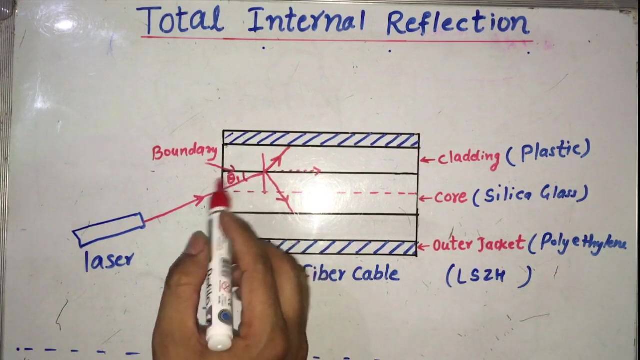 in the core. okay, so how it will be decided that whether this will enter to the cladding or it will move parallel to core cladding boundary or it will move back into the core if, for example, this is the angle of incidence at which ray of light enters to the optical. 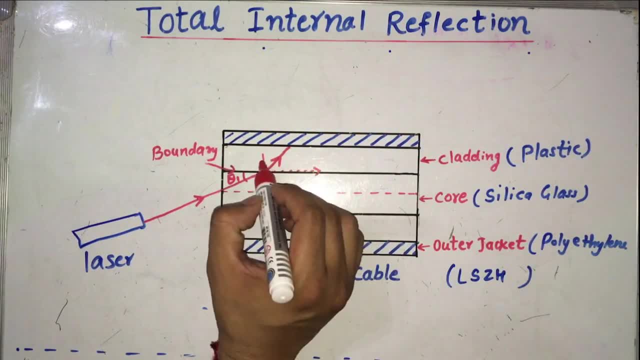 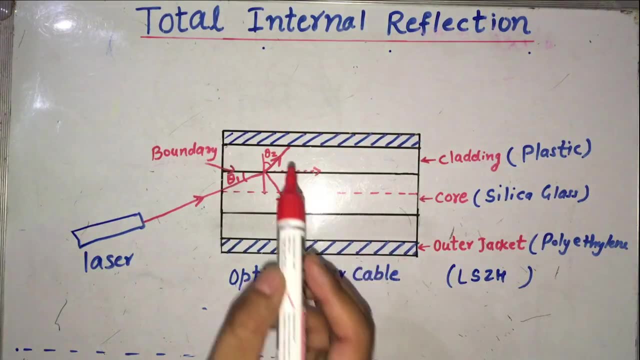 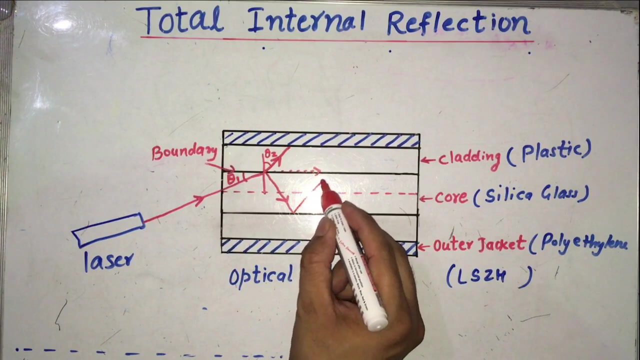 fiber. okay, and this one is the angle of reflection, theta 2. so total internal reflection is if a ray of light enters to the optical fiber and, after striking through the core cladding boundary, it returns back into the core and keep on reflecting again and again like this. 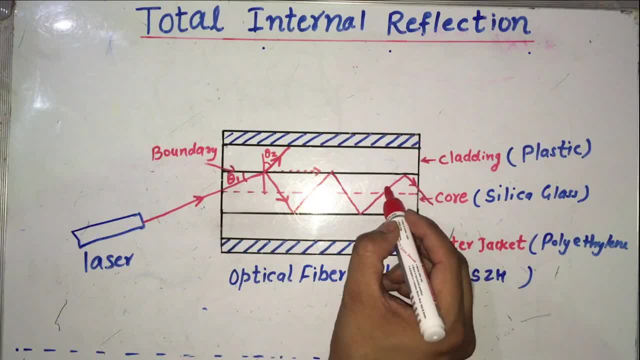 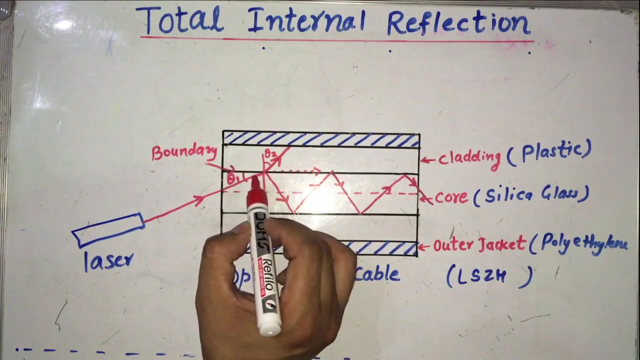 and reaches to the second end of optical fiber, then this phenomena is called as total internal reflection. but for the total internal reflection to takes place, there is a condition for this angle of incidence and there is a law called snell's law, which describe the relationship between angle of incidence and angle of reflection when light passes through the boundary between. 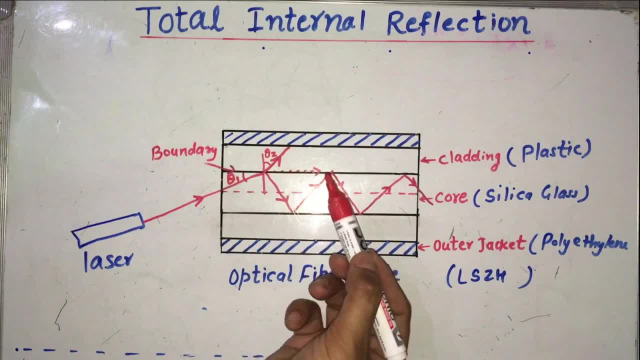 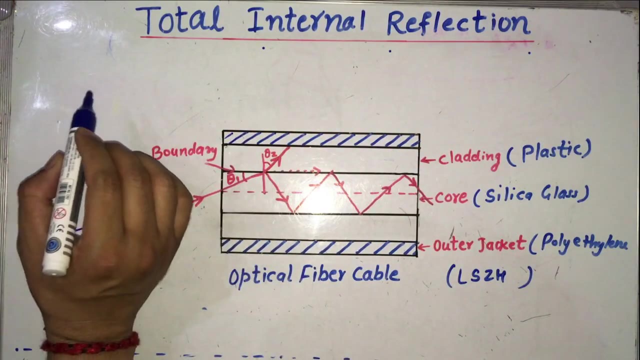 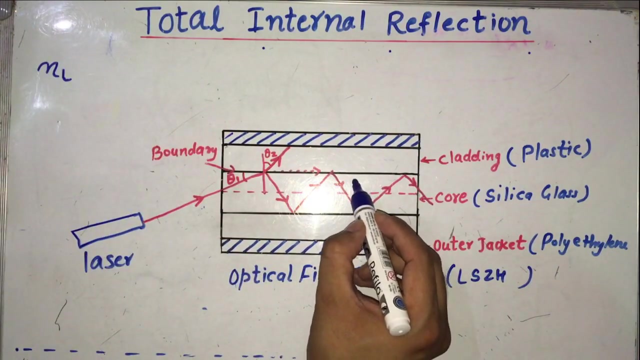 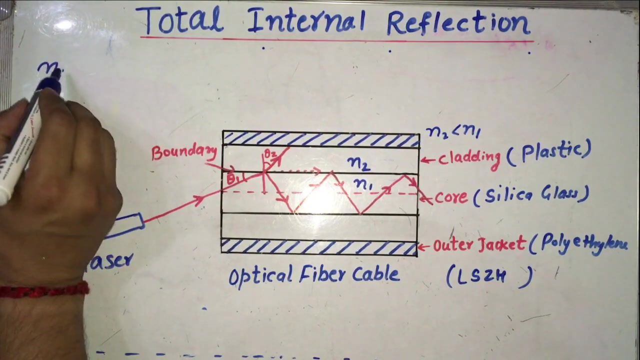 two isotropic mediums like water, glass, air or glass, silica or plastic. now let us understand this snell's law first. Now snell's law says that if n1 is the refractive index of one medium and n2 is the refractive index of another medium, where n2 is less than n1, then n1 sine theta1 is equal to n2 sine. 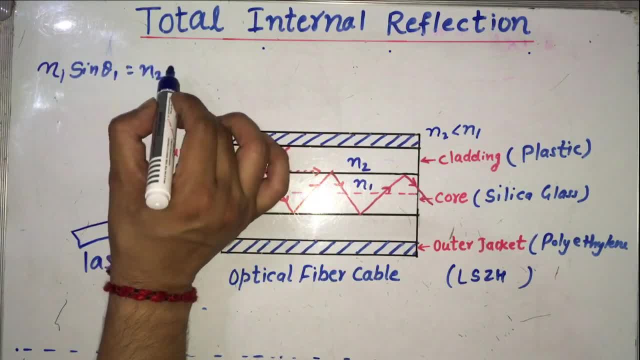 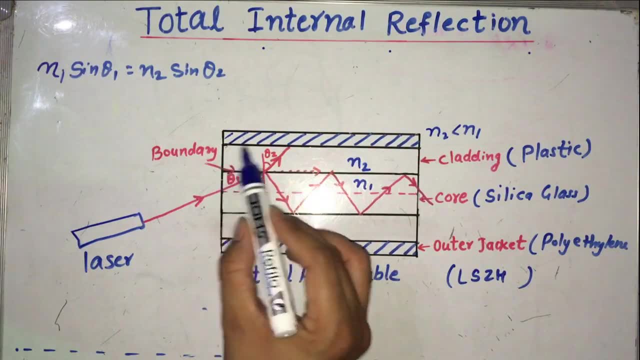 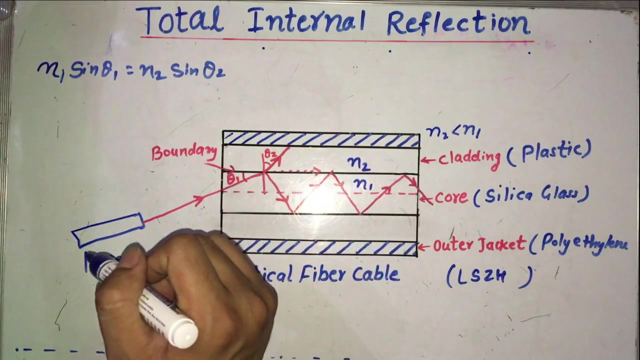 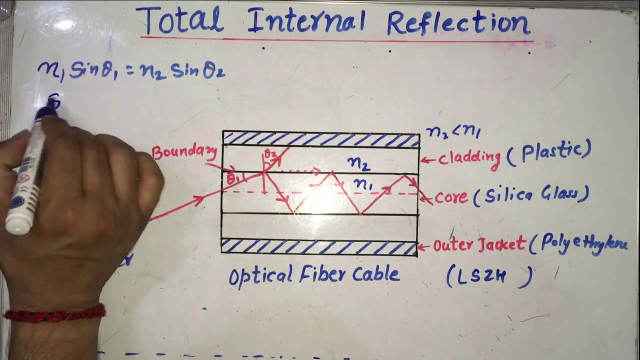 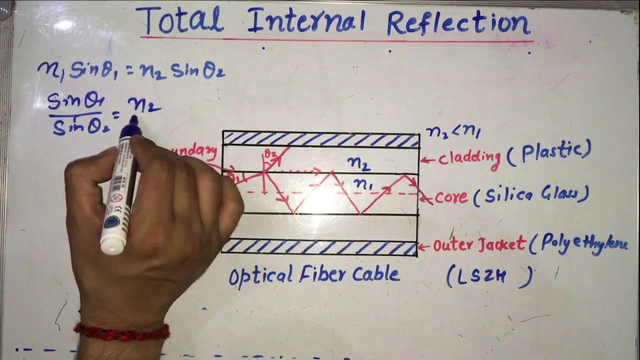 theta1. is equal to n2 sine theta2, and where theta1 is the angle of incidence and theta2 is the angle of refraction. Now light enters from the medium with refractive index n1 to the medium with refractive index n2.. So from here, sine theta1 divided by sine theta2, it is equal to n2 by n1. and from here, 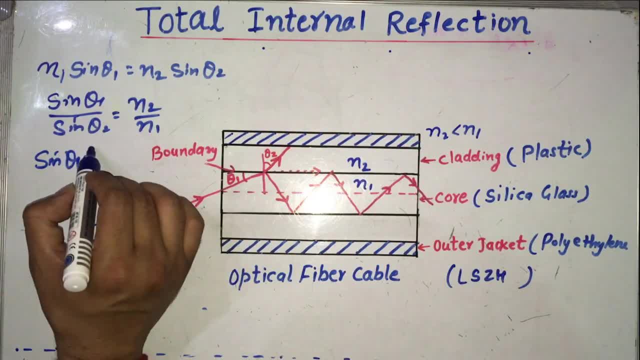 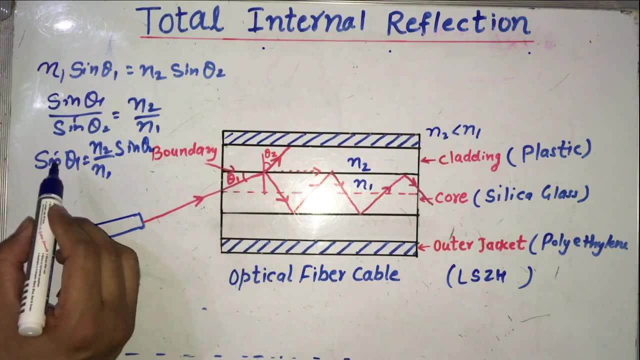 sine theta1, it is equal to n2 by n1 and sine theta2.. So from here you can see that the angle of incidence is equal to n1 and the angle of refraction is equal to n2.. We can find out a critical angle, theta c, which is the value of theta1, for which theta2 will be equal. 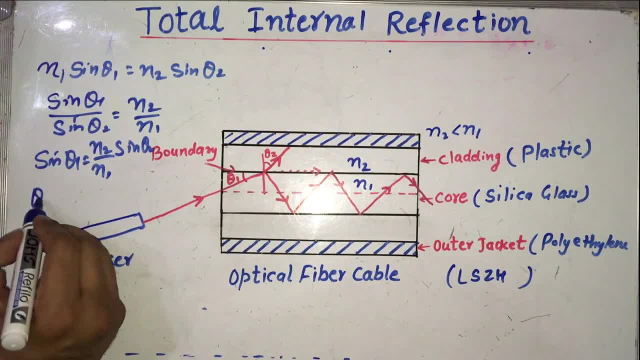 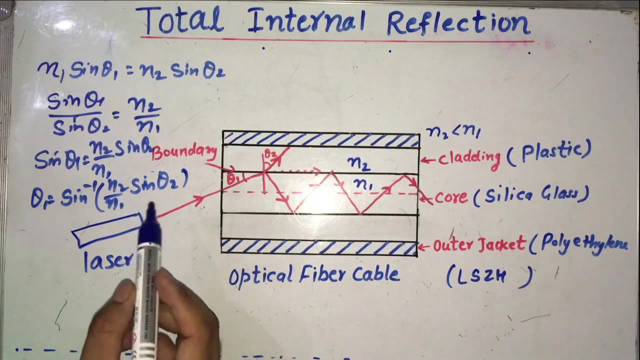 to 90 degree. So from here theta1. it is equal to sine inverse n2 by n1 and sine theta2.. So value of critical angle: theta c will be equal to sine inverse of n2 by n1, sine theta2, where this theta2 must be equal to 90 degree. So theta c will be equal to sine inverse n2 by n1, because 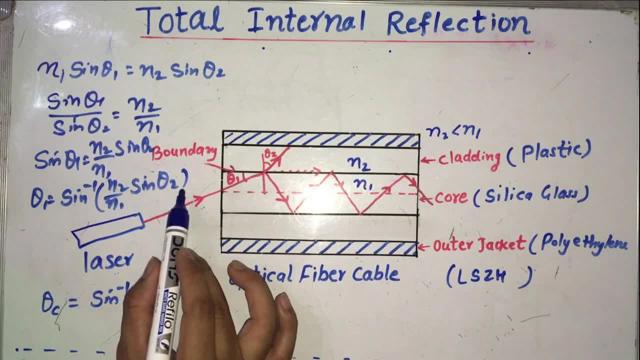 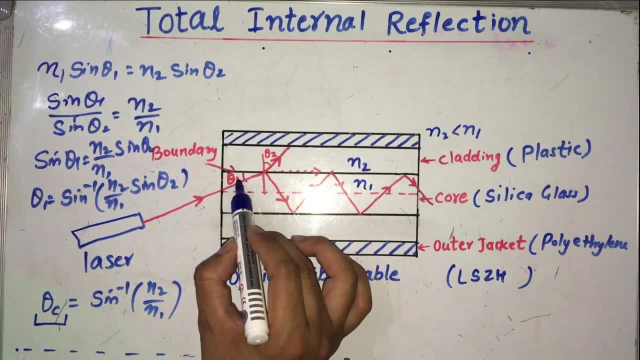 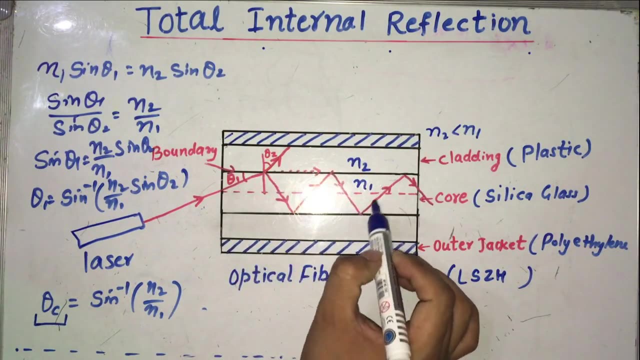 sine theta2 will be equal to 1.. If a ray enters from the medium with refractive index n1 to the medium, then it will be reflected back from the boundary of core cladding interface. So in other words, we can say that if theta1 is greater than theta c, then when a ray of light will enter this 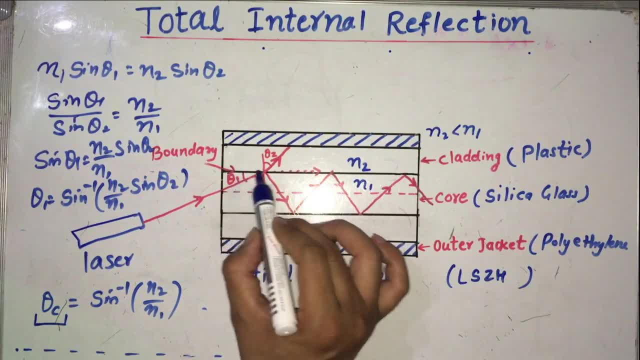 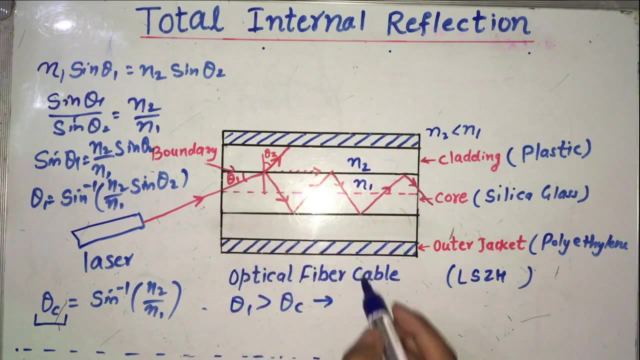 medium, then it will be reflected back from the boundary of core cladding interface. It will not reach the core cladding interface. So from here we can see that the angle of incidence theta1 is to the second medium. So this is the condition. when theta1 is greater than theta c, then the ray. 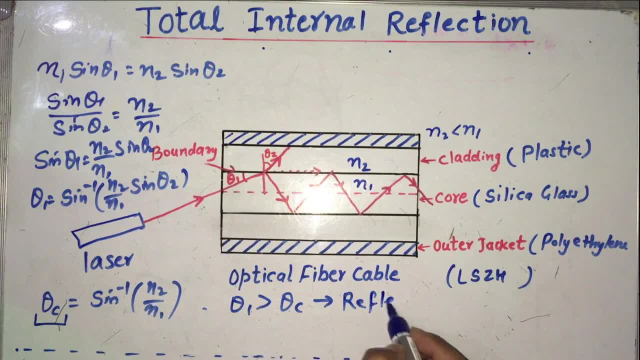 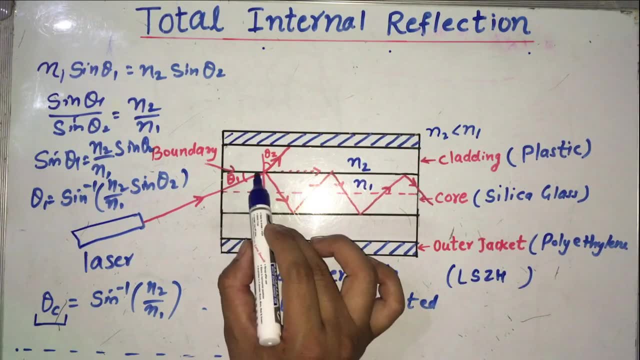 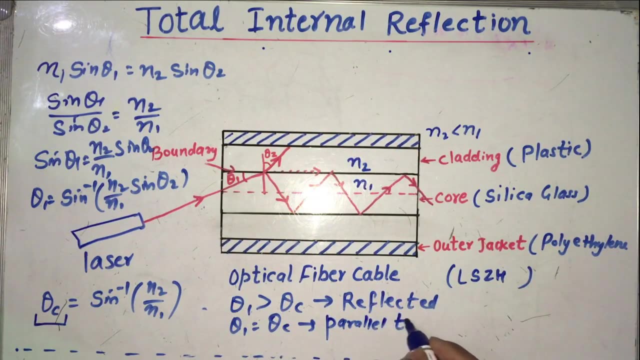 of light will be reflected. If this theta1 is equal to theta c, then ray of light will travel parallel to core cladding interface. So this is the condition: when theta1 is greater than theta c, then the ray of light will travel parallel to core cladding boundary. and third one: when theta1 is less than theta c, then the way the ray of light will be refracted to cladding medium. 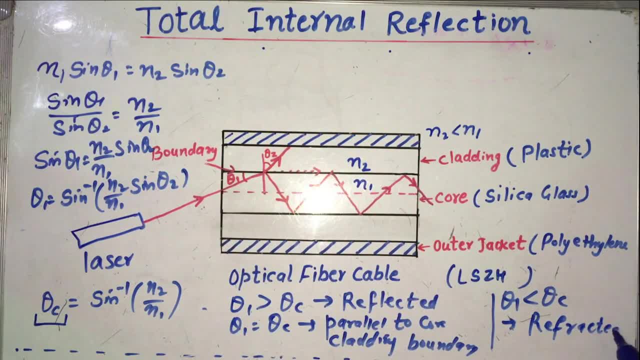 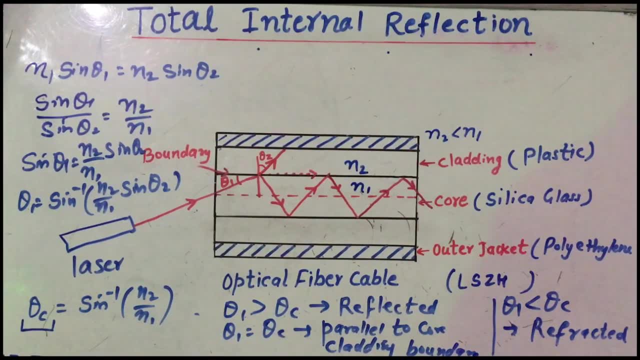 So, for example, we want to calculate, for example, we want to calculate, for example, we want to calculate a critical angle for a ray of light which is moving from water to air. a critical angle for a ray of light which is moving from water to air. 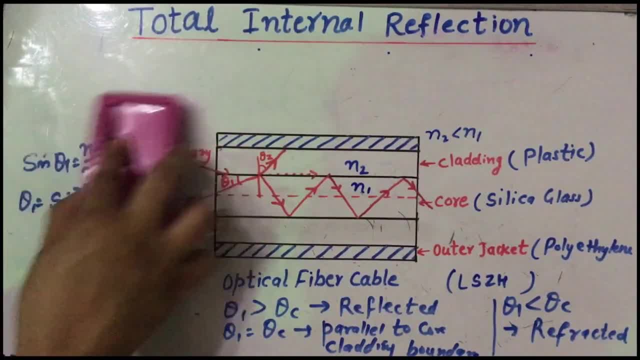 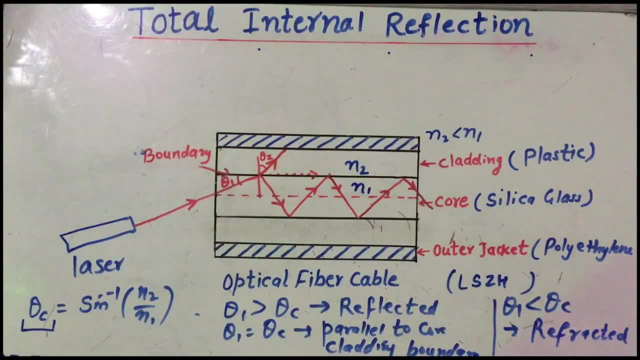 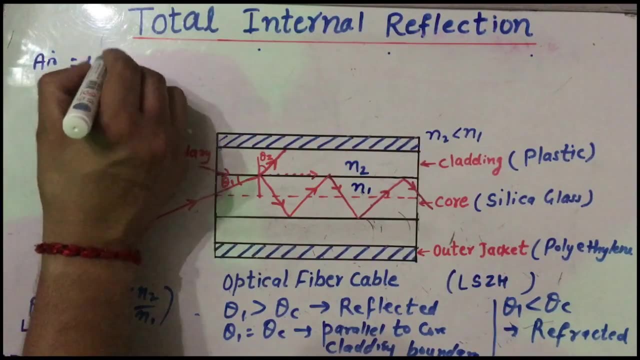 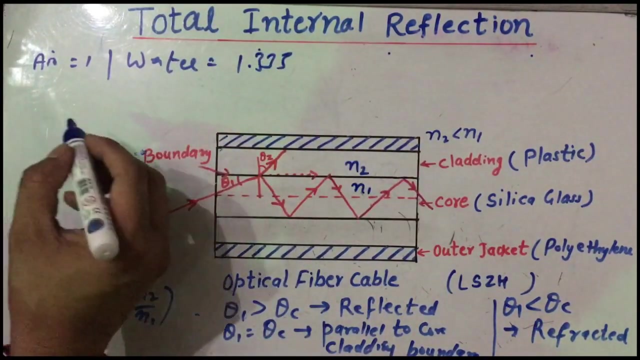 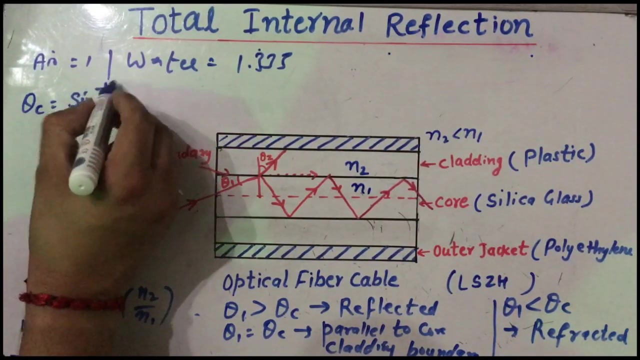 So let us take this example and understand it. that how we can calculate this angle. So refractive index of air is 1 and refractive index of water is equal to 1.33.. 333, okay, so theta C, that is critical angle. it is equal to sine inverse of 1. 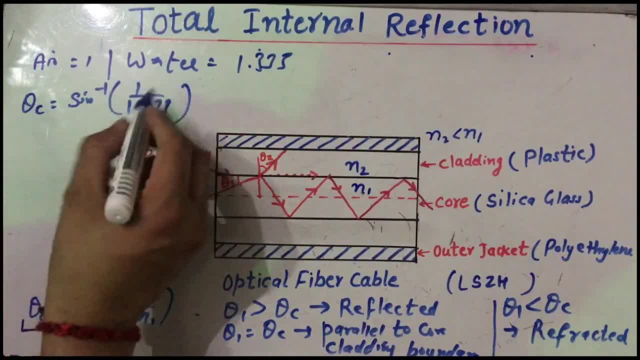 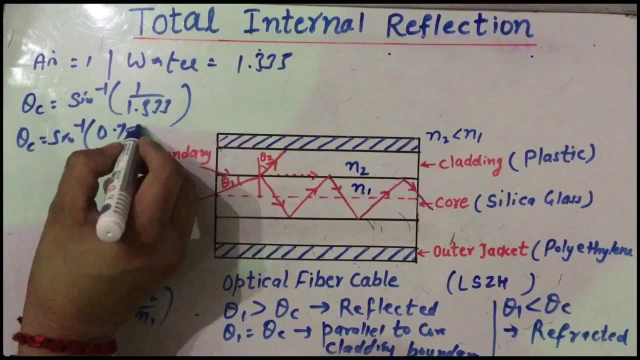 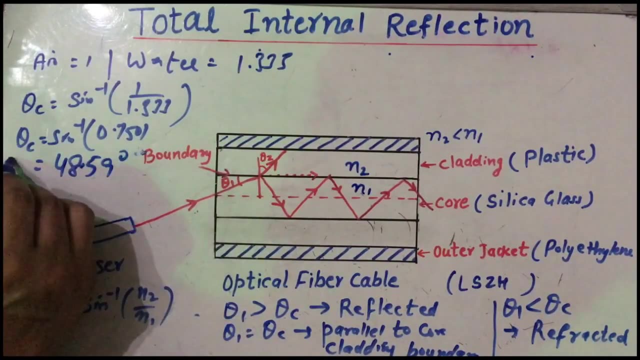 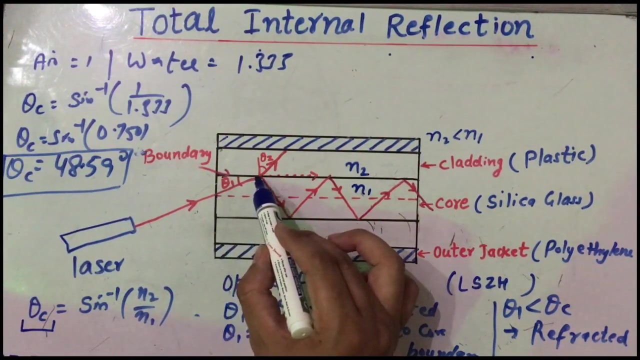 by 1 point 333, so it comes out to be sine inverse of 0.750, which is approximately como 48.5 x 5, 9 degree. so any ray of light which will incident upon this boundary at an angle which is greater than 48.5 nine degree, that will. 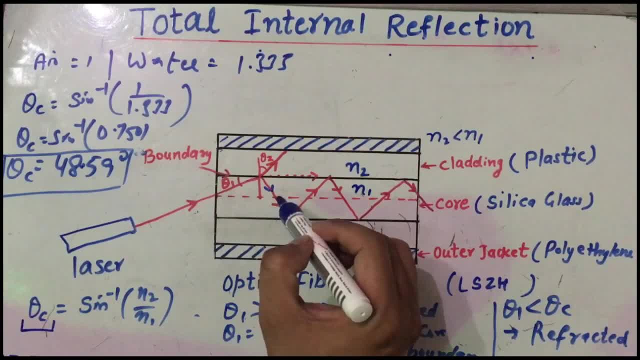 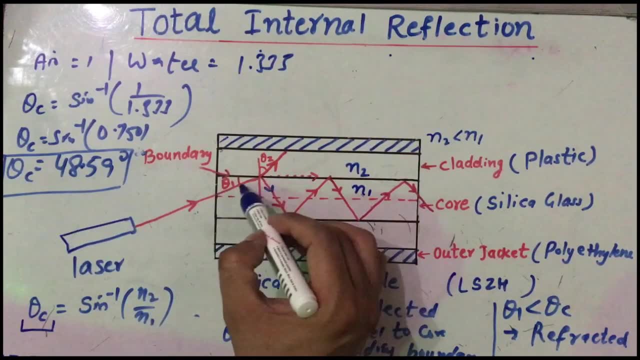 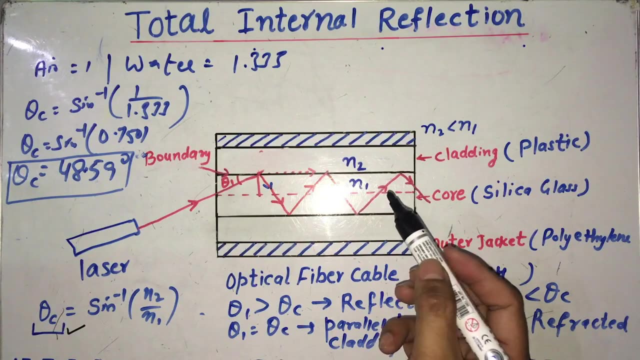 be reflected back into the medium, and if the angle of incidence theta 1 will be less than 40, eight point five nine degree, then that will be 한데 reflected through this. okay, i hope now you have a better understanding of what is refractive index. 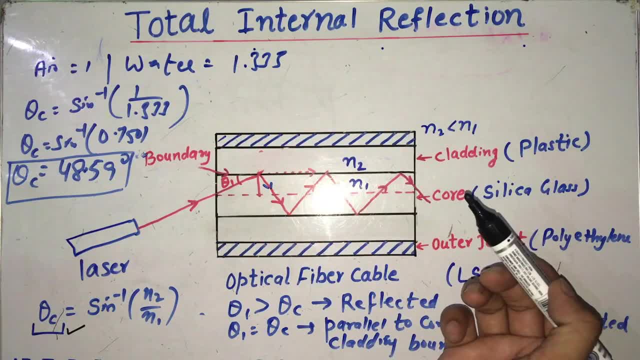 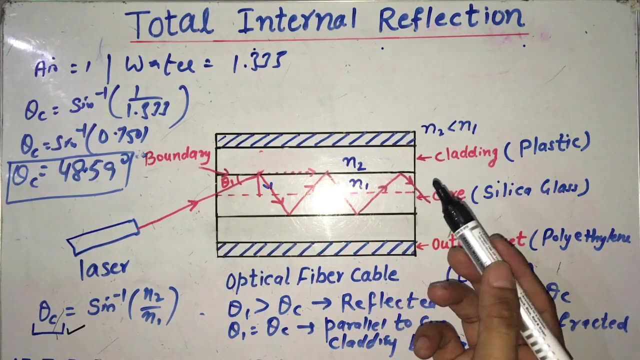 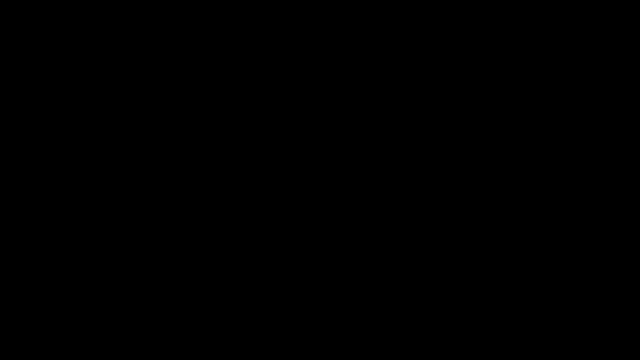 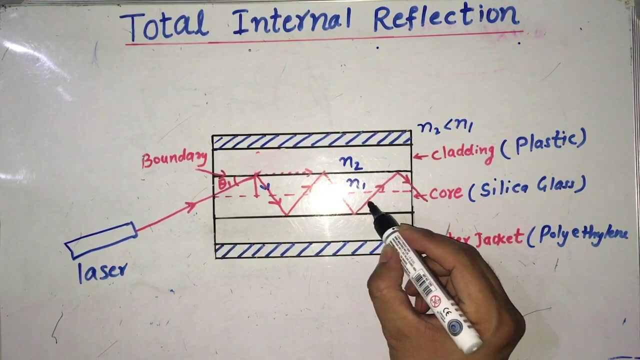 snell's law and, ultimately, total internal reflection. if you have any queries related to total internal reflection, then you can comment me in the comment box. thank you you. 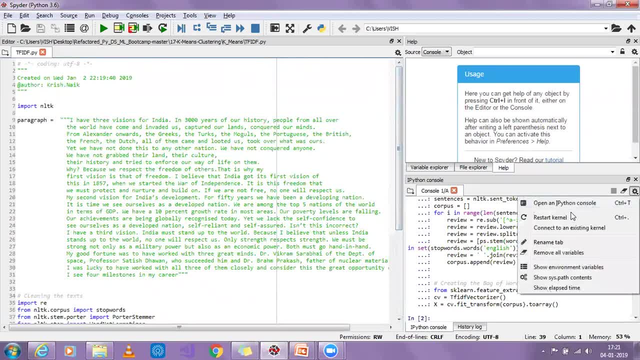 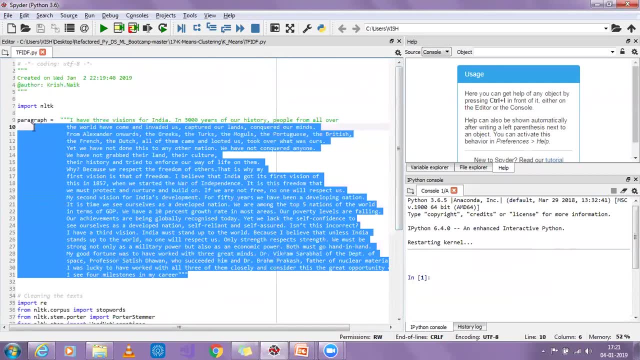 And I'm going to use the same NLTK library. So first of all, let me restart this kernel. The paragraph that I'm taking is from the same example that we have done in the previous stages. Guys always remember, try to understand this scenario, because after some videos, 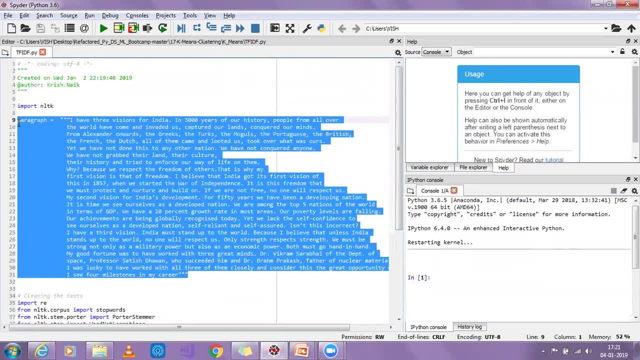 I'm going to upload a use case where we'll be doing sentiment analysis on restaurant reviews, or it may be on Amazon comments- right Comments on the product. We'll be doing a sentiment analysis and we'll be trying to find out whether it is a positive sentiment analysis or a negative. 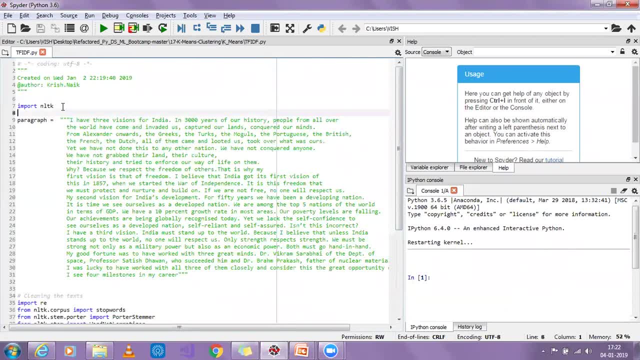 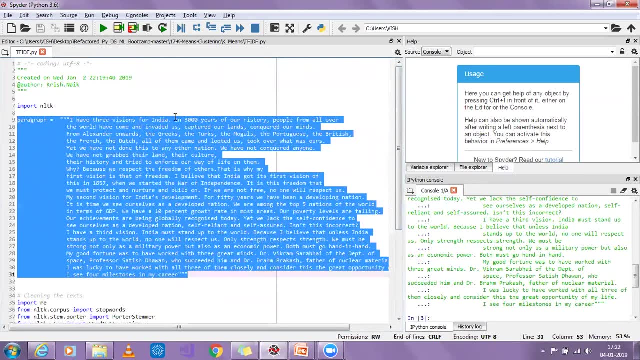 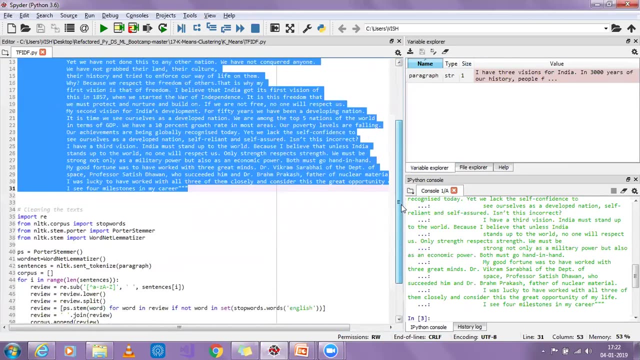 sentiment analysis Now with respect to TF idea. first of all, I'm going to import the NLTK library. Then I'm going to import this paragraph. Okay, My paragraph is got imported. I can see the paragraph here. Okay, Again, the first step is basically cleaning the text, Always remember. 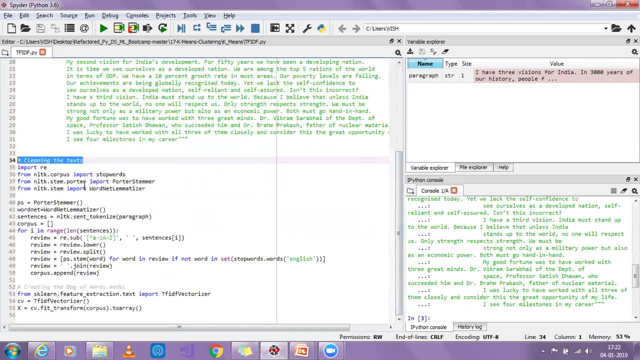 I have to clean the text And I've already explained why we have to clean the text. For cleaning the text, what I'm going to do: I'm going to import the NLTK library And I'm going to import the NLTK library And I'm going to import the NLTK. 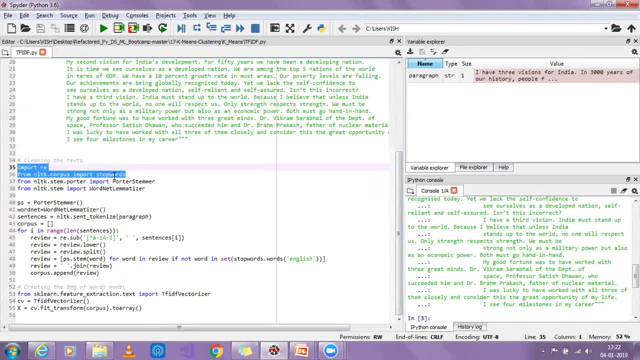 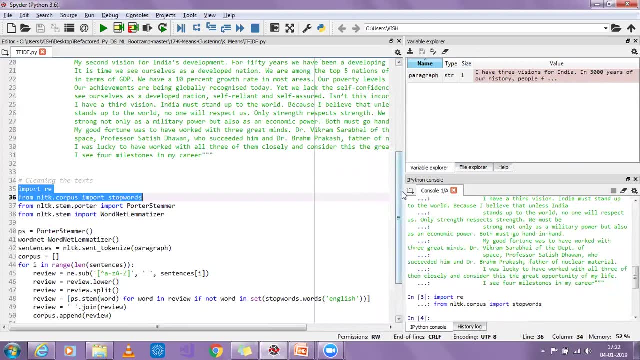 regular expression library. I'm also going to import the stop words. Let me just zoom in. So this is my stop word and regular expression which I've imported. Okay, Then, what I'm going to do is that this library is basically for stemming purpose.